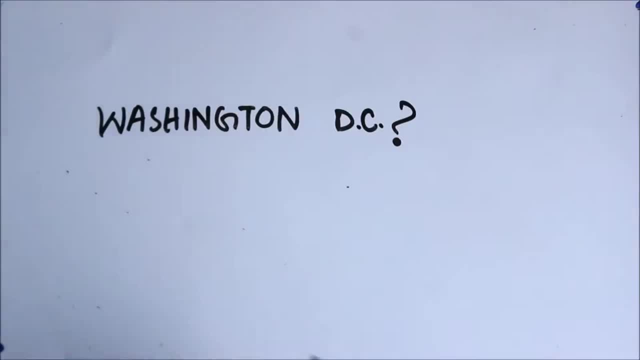 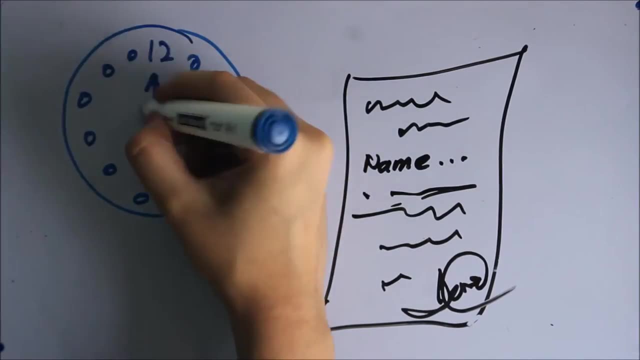 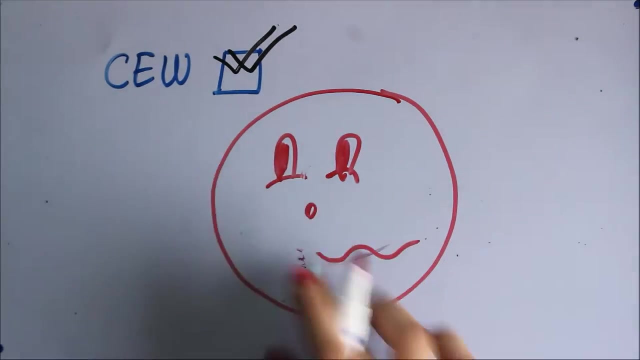 extremely excited about the idea of going to Washington DC for one whole week. Therefore, I decided to apply for it. But like any other major procrastinator and distracted by a million opportunities of a high school student, I sent in my application just minutes before. 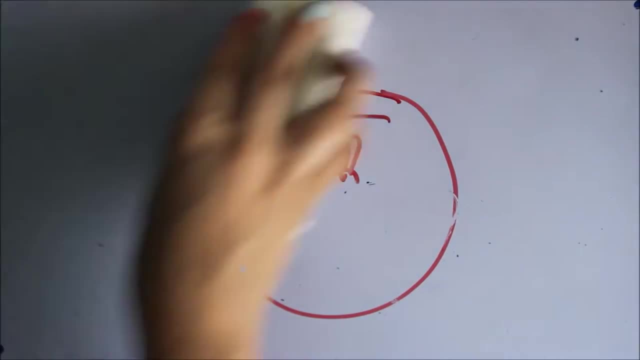 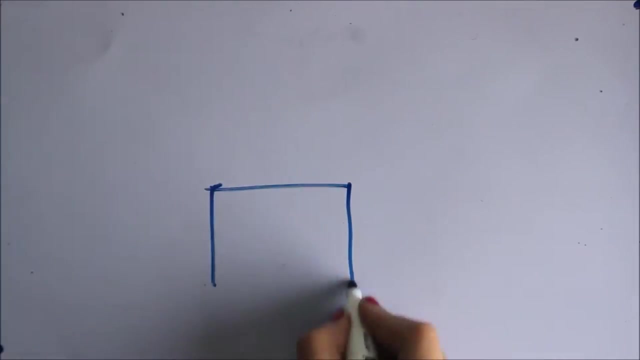 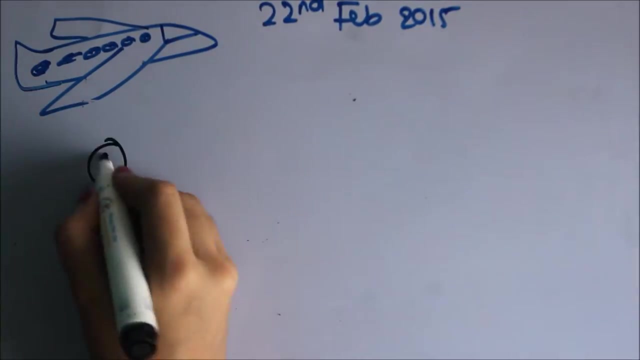 the deadline and I was pretty nervous about the results. However, to my sweet delight, I got the confirmation email of my selection somewhere in January, and I cannot even describe how happy and proud I was to see it. It was February 22, 2015 when I arrived in Washington DC. I met some old friends while 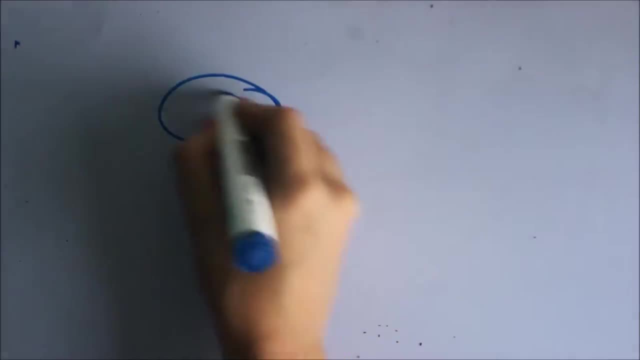 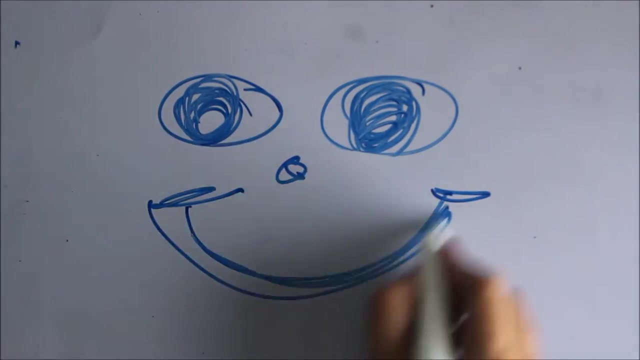 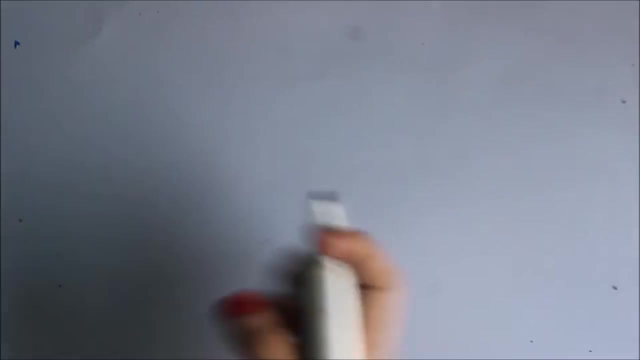 making a whole lot of new ones as well. I was so thrilled about getting started that I could barely even sit still. To be honest, I had no idea that I could be this excited about something before. When I got my hotel room keys, I found out that I was to share a room with three other. 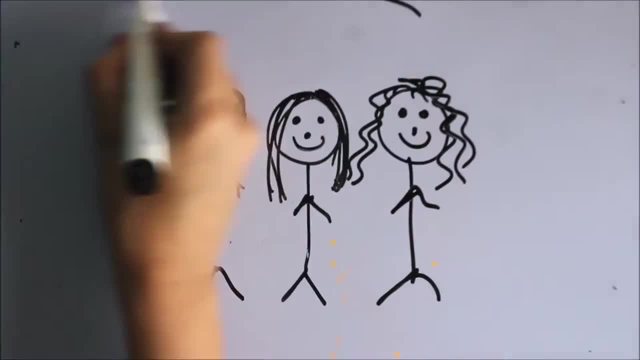 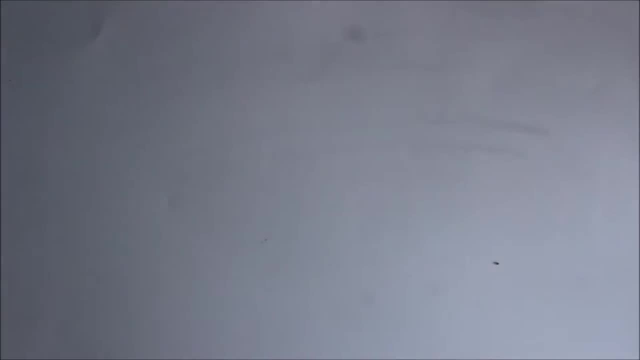 exchange students from Palestine, Egypt and South Africa. I was really happy about this, because I had actually never even met people from these nationalities before I got here. Anyways, CEW turned out to be a very fun and beneficial place for me to spend my time. I 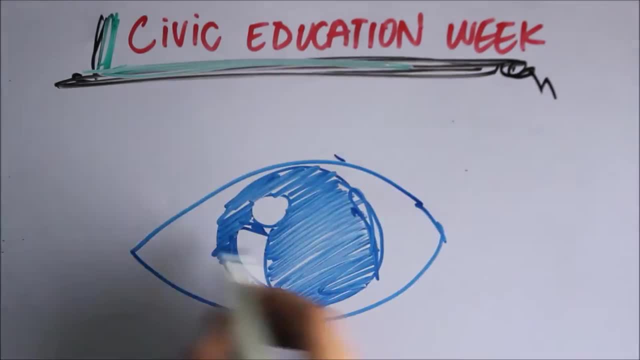 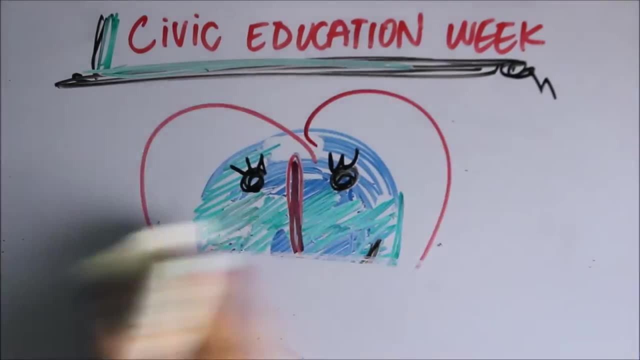 really enjoyed it. CEW was a very exciting conference. It exposed us to a variety of perspectives about pressing issues happening across the globe in a friendly and accepting manner. It taught us to respect diversity and act as peace builders in our communities and the world at large, And we 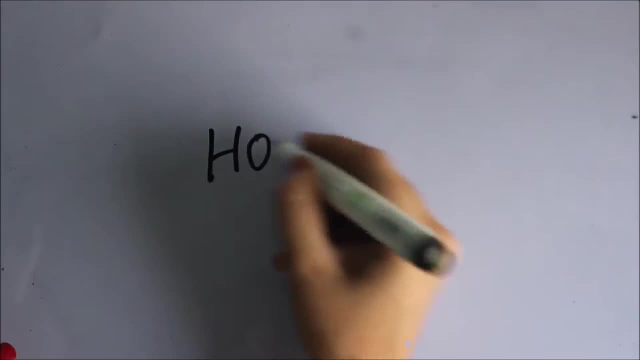 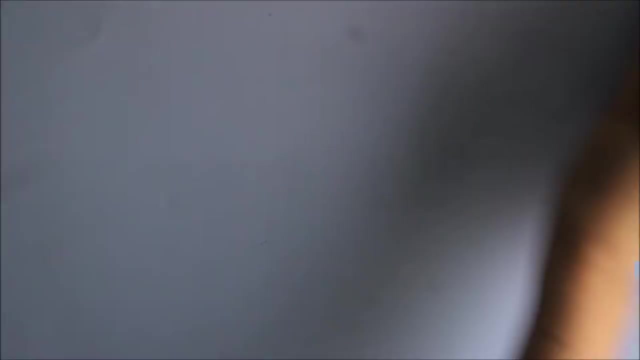 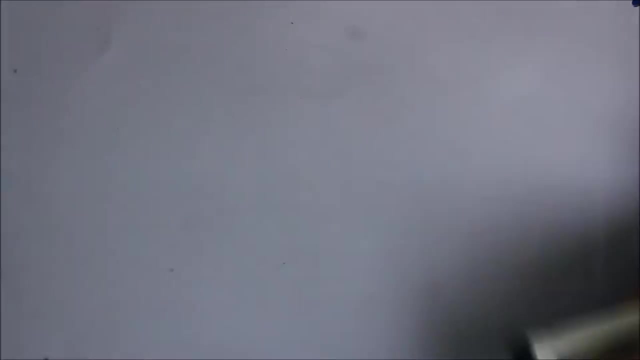 had a sense of pride in learning these things because of the way they were taught to us in CEW. Unlike normal conferences, CEW did not happen within the confines of four walls of the University of Washington DC or consisted of a zillion selfies only. We were always moving around and our conference 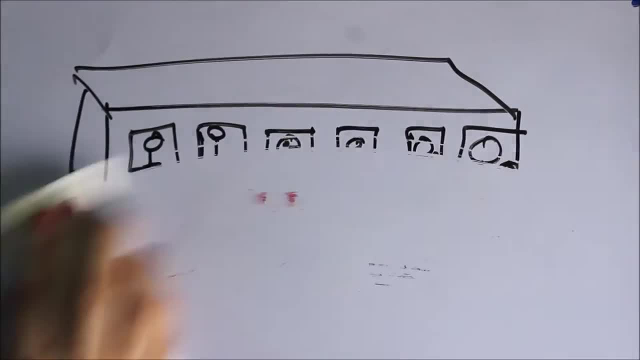 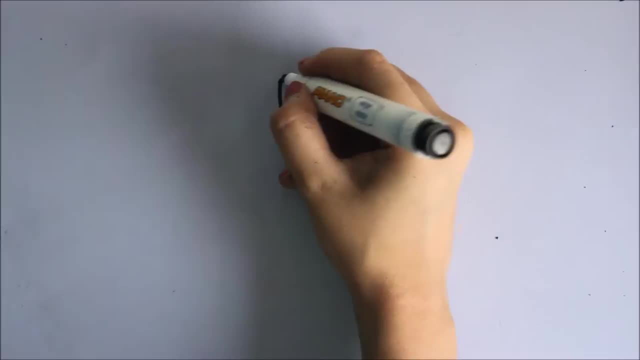 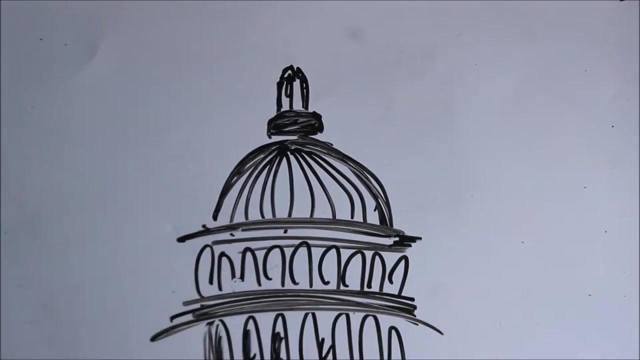 sessions happened basically anywhere from our tour buses to the Washington streets, museums, memorials, the US State Department building to the government buildings of the breathtaking Capitol. Washington DC became our classroom and its history became our curriculum. There was just so much to learn, to do and to see. 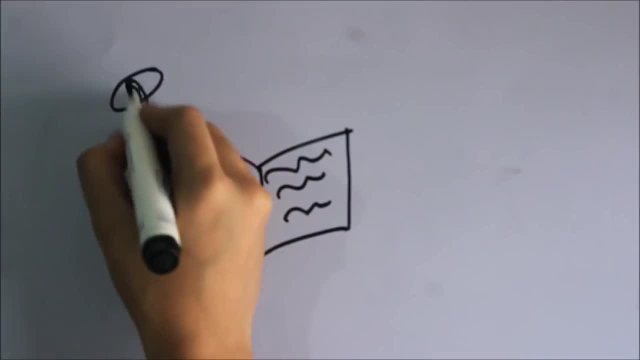 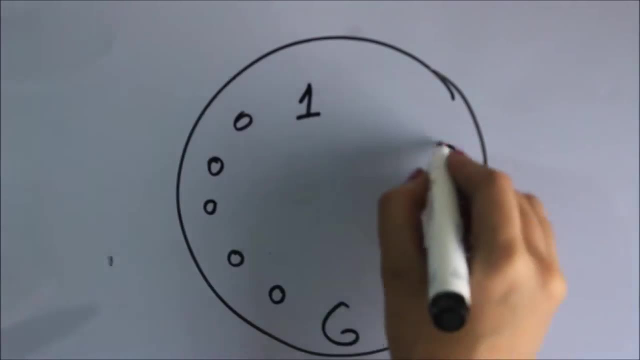 I was so excited to be here. I was so excited to be here. One thing is for sure: CEW has one of the most jam-packed and concentrated schedules I had ever experienced, And the good thing is that it taught me to be more. 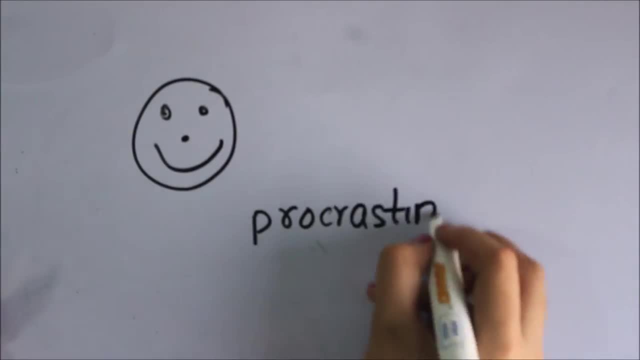 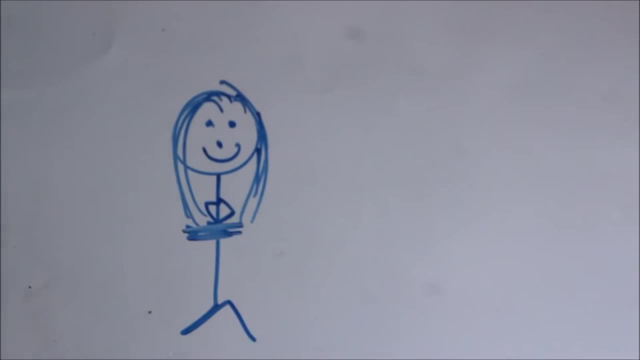 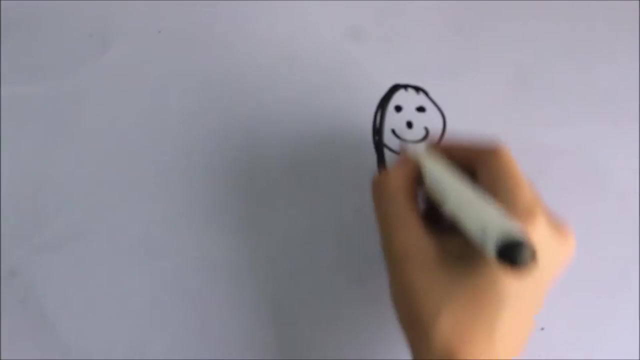 alert and manage my time and things better and not procrastinate. So time management- That's one of the many leadership qualities right there. A huge part of the CEW experience was learning how to become a better leader and stand up for others. 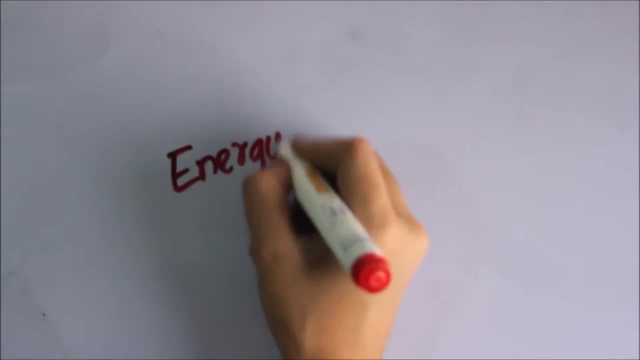 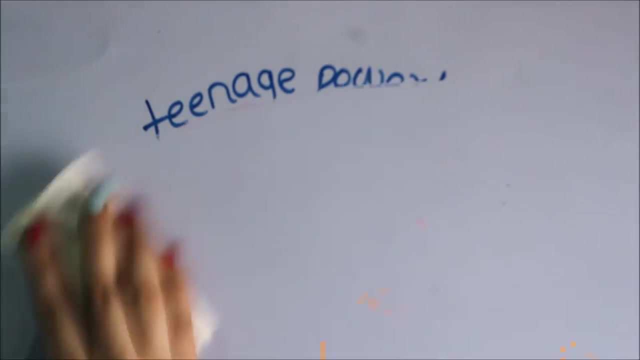 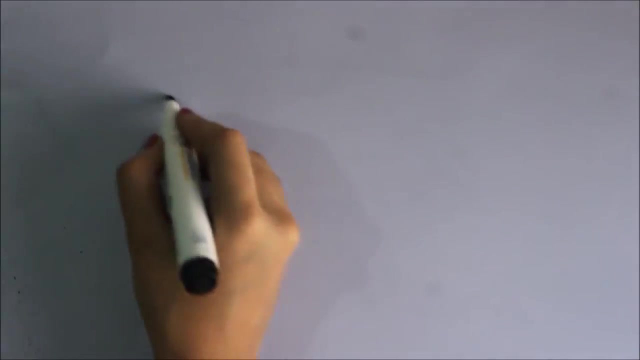 We as teenagers are so full of energy and enthusiasm and CEW taught us to take good ethical initiatives to shape this enthusiasm in helping our communities and put that teenage energy supply to a bigger use. Being a part of CEW definitely gave me the confidence and determination to return to 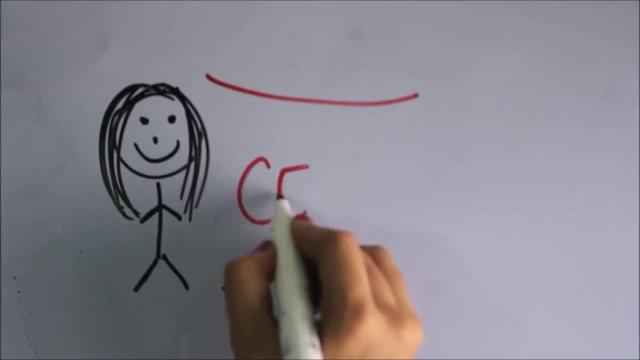 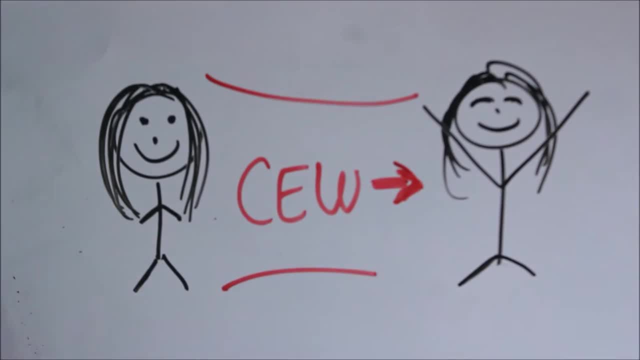 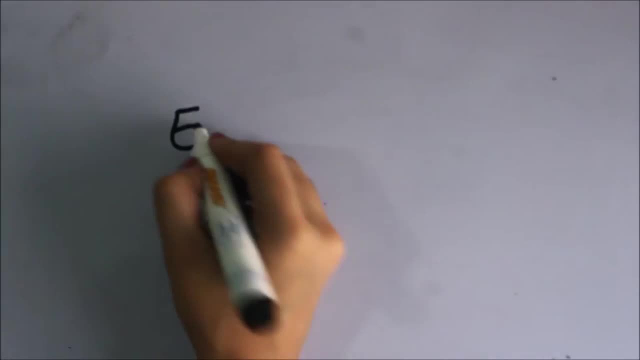 of projects. I participated in a number of projects. I participated in an initiated numerous community service projects in my hometown. with that same spirit, Looking back onto my exchange year, CEW stands out to me as one of those memories that will always remain close to my heart. 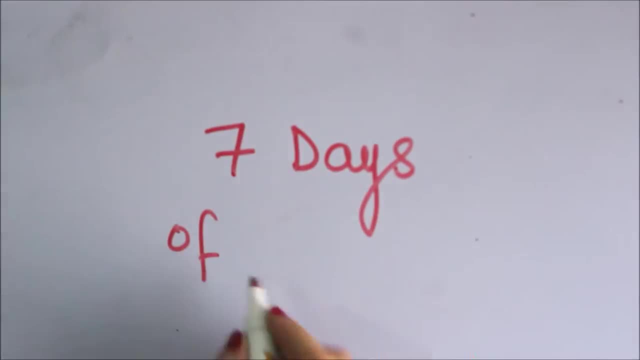 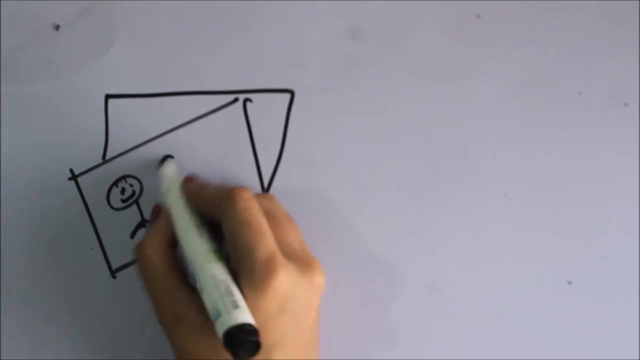 It was just a matter of seven days, yet we learned so much about America, the world and ourselves. I think CEW is an experience that stays with you for the rest of your life. It stays with you in the form of the friends that you made, the memories that you collected, the lessons you learned and the way you will perceive the world. 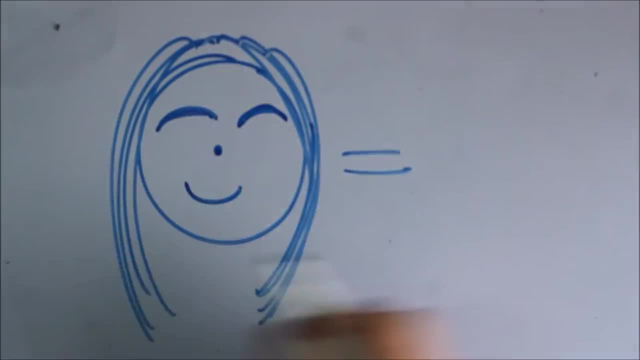 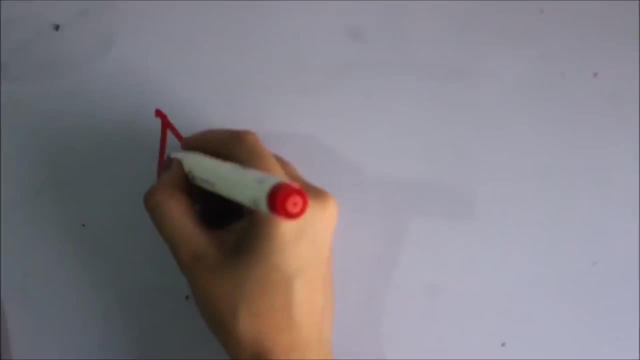 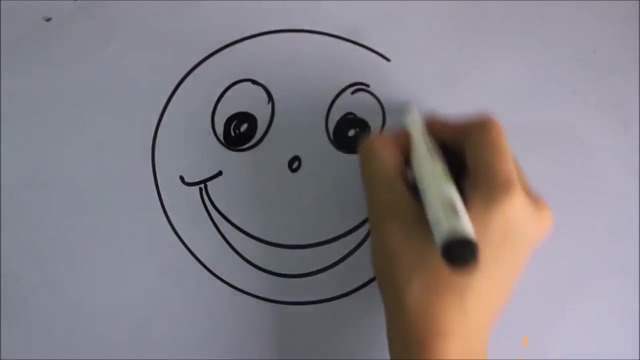 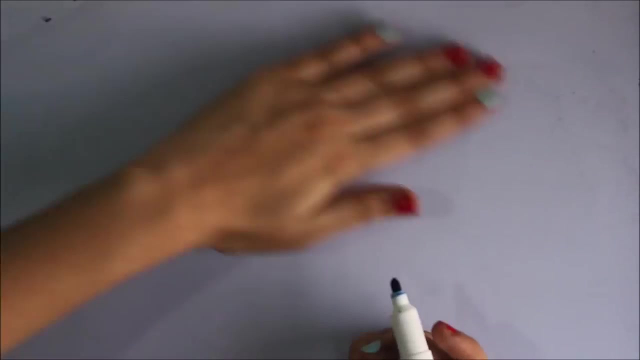 And I am extremely glad that I could be a part of CEW. You know, if I could go back in time, there is not a single thing I would change about my CEW experience. It was beyond perfect. So if you happen to get selected for this awesome conference, know that you are in for the most amazing week of your exchange life.